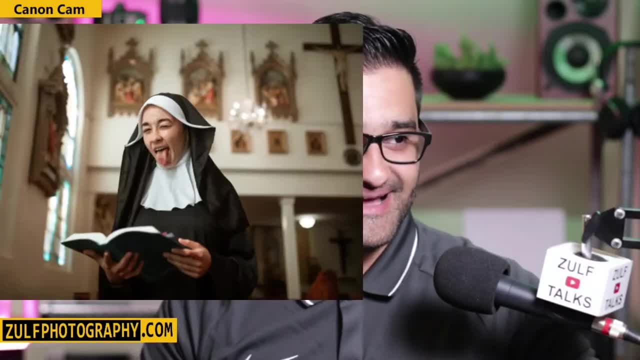 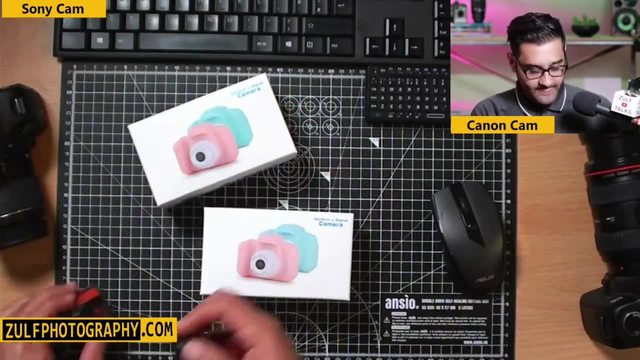 And we have got a multi-camera setup. So glad you like that Greedy nuns- Amazing name, by the way, Sick name Got memory cards lined up. You know I'm hoping we are good. So yeah, Now these, My god. 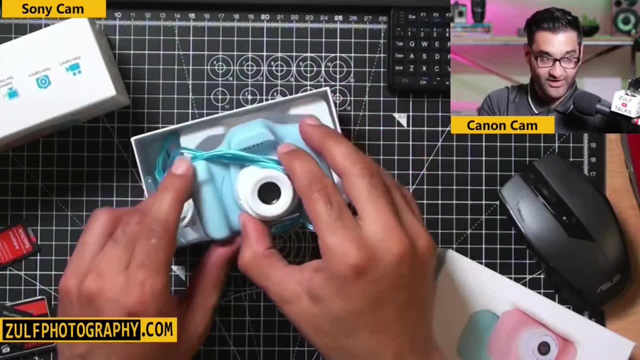 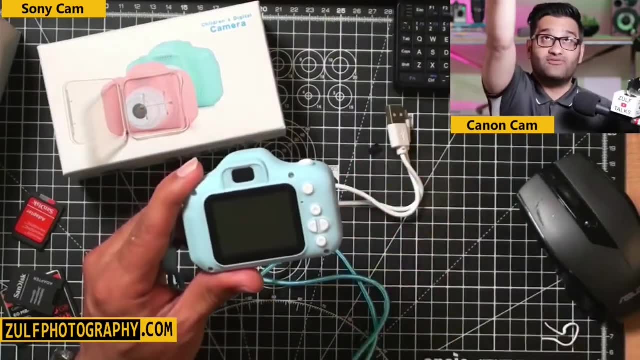 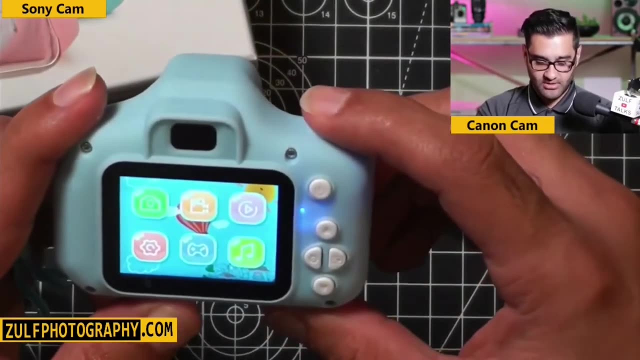 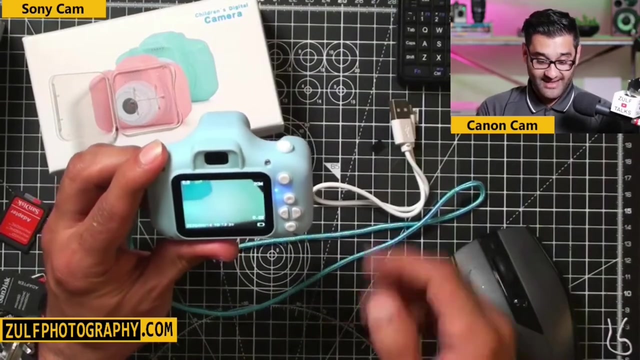 I'm using it. I'm definitely using the wrong tool, Because it's never designed for kids. Oh my god. So now the moment of trust comes on. Oh my god, It's like kids getting a present. Okay, Oh, okay, That should picture one. Oh my No way. You know what 20 megapixels, mate, That is. 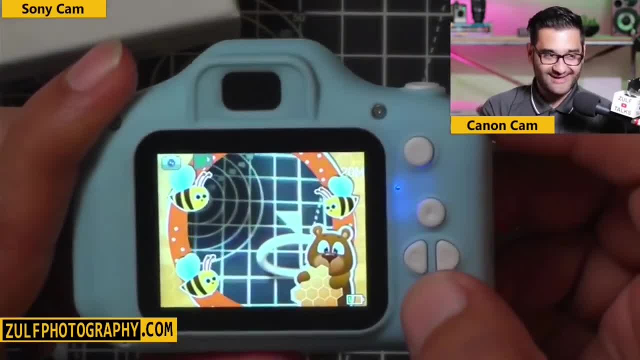 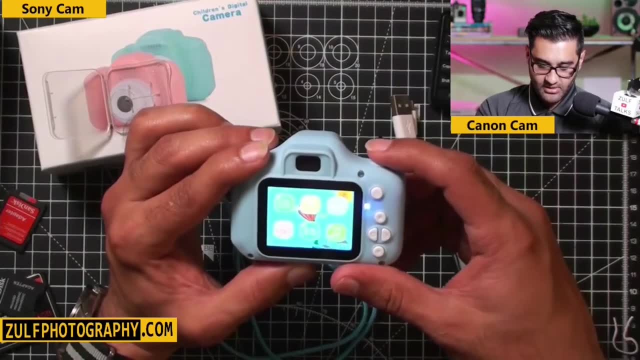 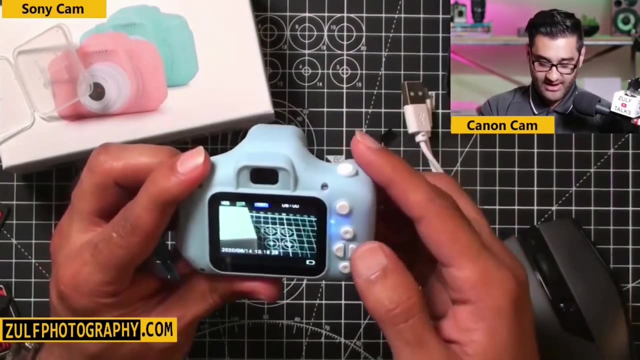 comparable to a mobile phone. You've got a little That is just Imagine a little kid walking around taking photographs with a mini DSLR. Accept that, Okay, 720p. A little video recording. I'm going to test the video recording as well, So let's see. 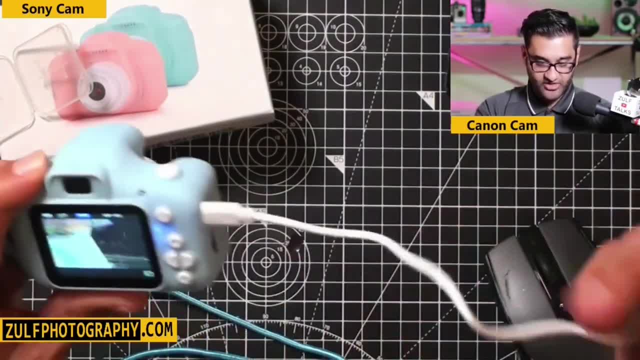 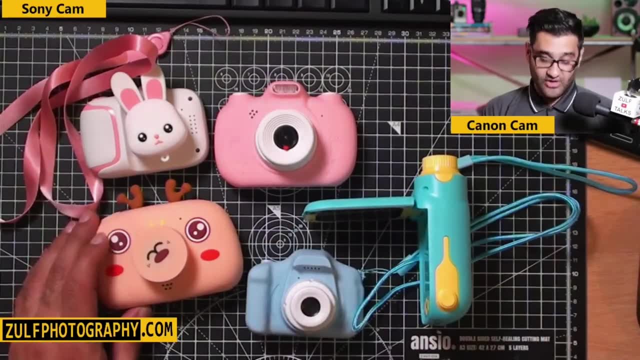 Because I reckon we need to charge this And I probably can take the files off at the same time as charging it. Okay, So if your series is about photography And you want your kids to get a little gift idea, There's a number of cameras there. You can see from the small and cute. 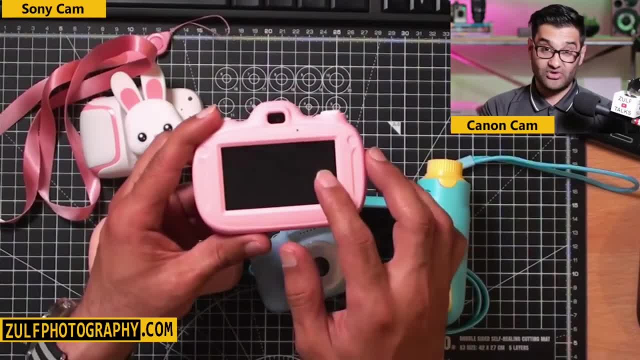 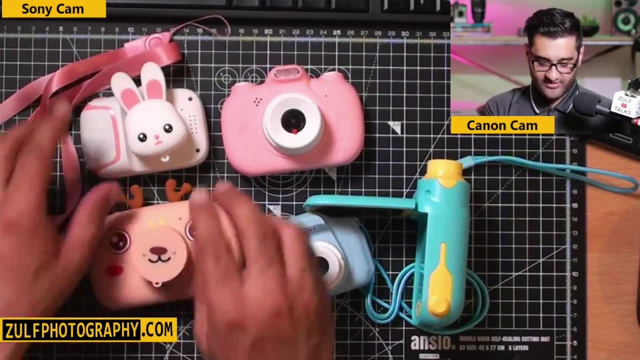 To the small And actually quite decent That has a touch screen on it And it's actually got games options. here You can see they have little cute lens caps Like that reindeer face is one And obviously we've got a rabbit one there, So we've done a couple of testing on this. More of a camcorder. 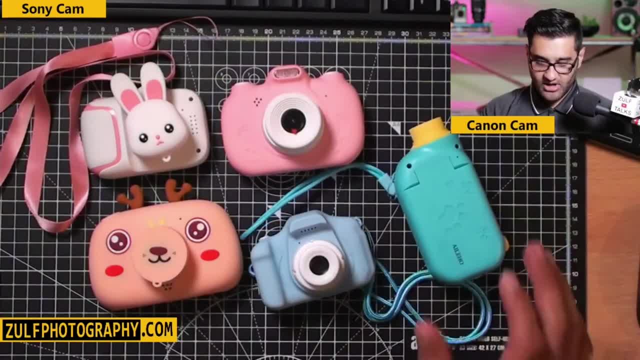 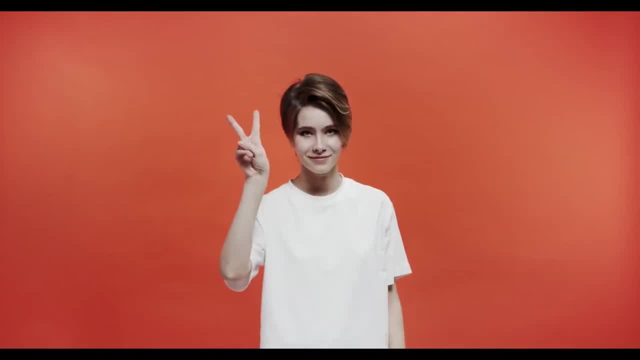 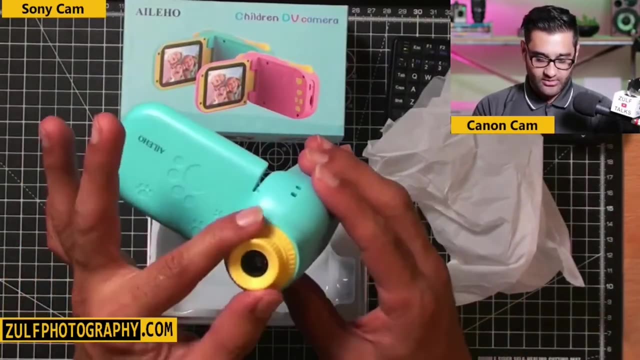 style one here And you can see these are all little options for you to get shooting basically photos, Even video and games as well. That box open, Okay, So nice solid box than I was expecting. It's got a nice little paw print, So okay. The lens can't be adjusted. 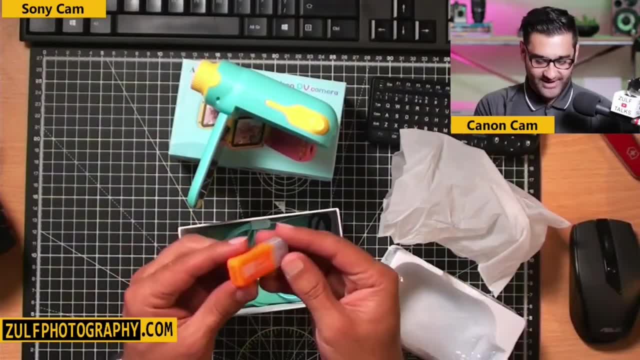 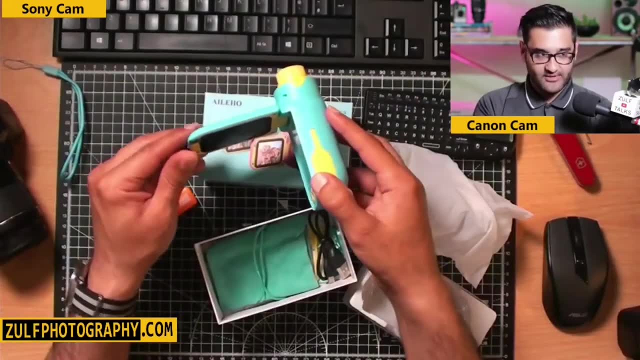 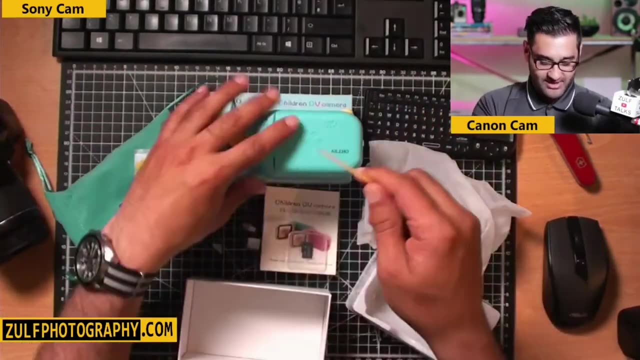 Oh, This one comes with a bit more people. So basically you plug a USB in, You put your card in the back. It's a micro SD card, Lipsight, Remember. it does not rotate. Keep it nice and scratch free. Okay, So that's that sorted out, And then probably feed it through. 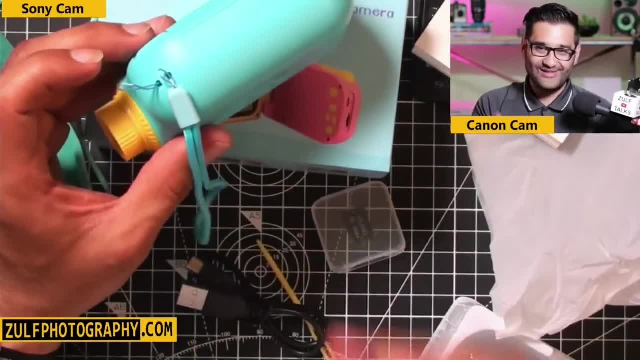 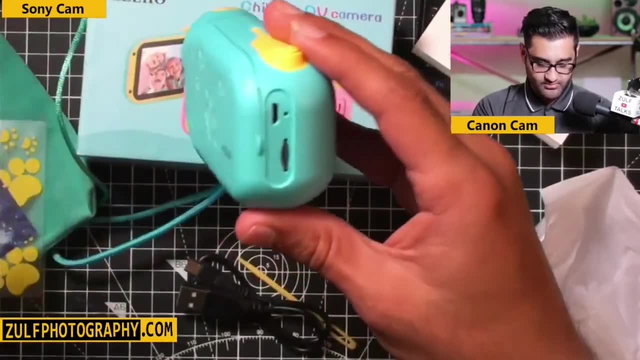 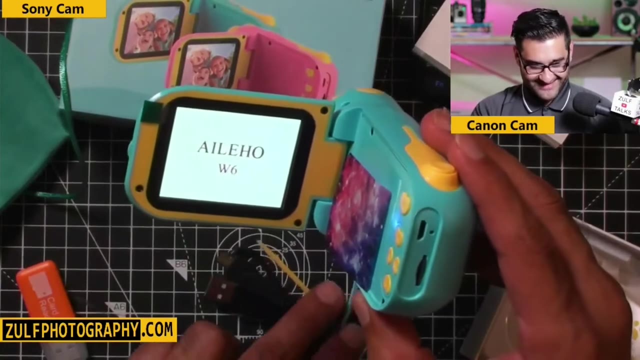 this: Wow, Look at that, Look at that. Okay, So now it makes sense, But they didn't tell you that in the guide. Just so you're aware. You know, Yep, So that's banged in. I wonder why that was not pre-stuck. Oh, Oh, People get ready. This is where it's all going to be. 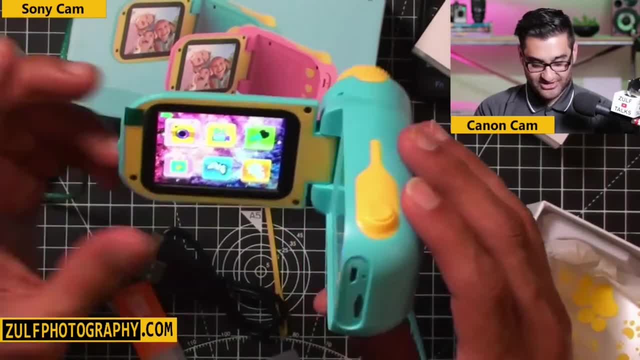 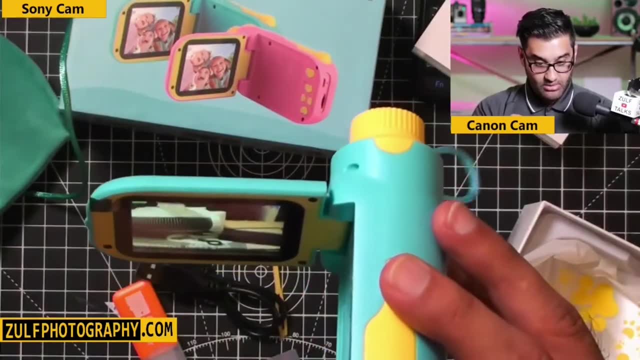 Make or break it now. So we've turned the camera. Whoa, I'm touching the screen again. Okay, One minute. So we're going to use the menus. Whoa, Wait a minute. Wait a minute, people. That doesn't. 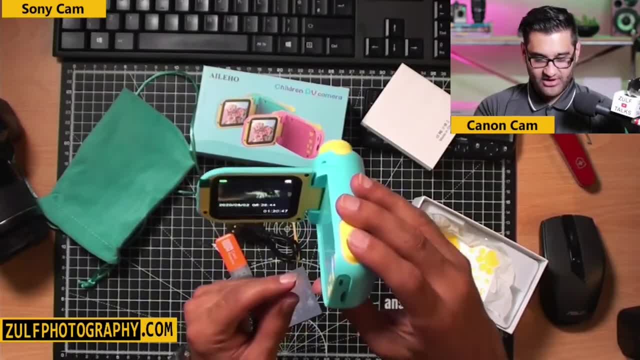 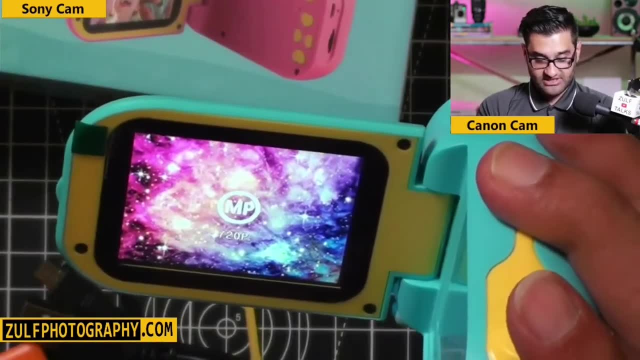 look too shabby, Okay Video. Ooh, That looks a bit A bit Juddery. Let me check settings and see if I can make that a better quality: 1080p, 720p, VGA, 1080p. So it does video in 1080p, Okay. So let's go back to the menu. 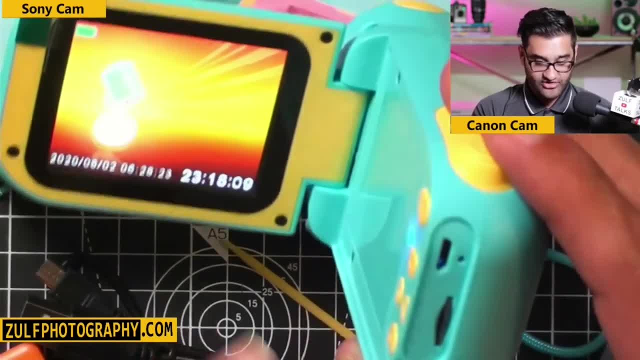 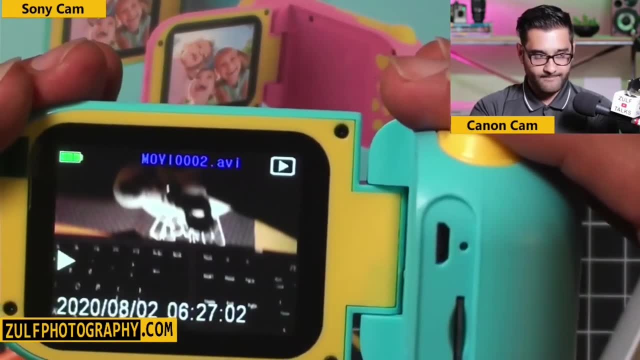 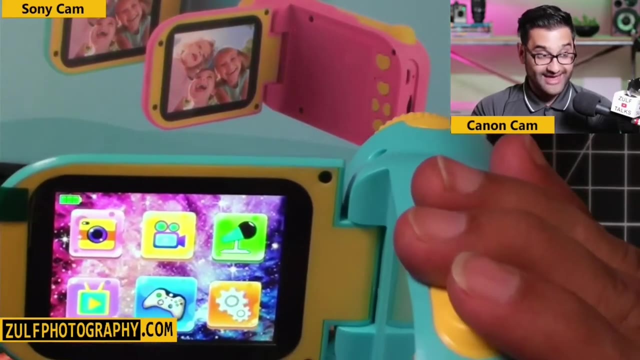 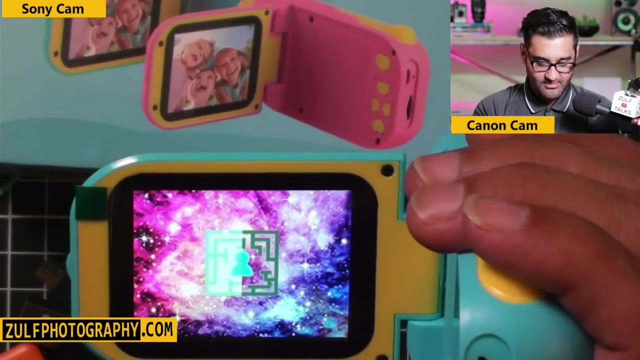 Recorder Whack. Okay, So that's the sound recorder. Let's go back Look at them. photos: Oh Choppy, Okay So games, Ooh, Games, Snake, Same as the push the box Maze of some sort. That is That game is actually. Let me have. 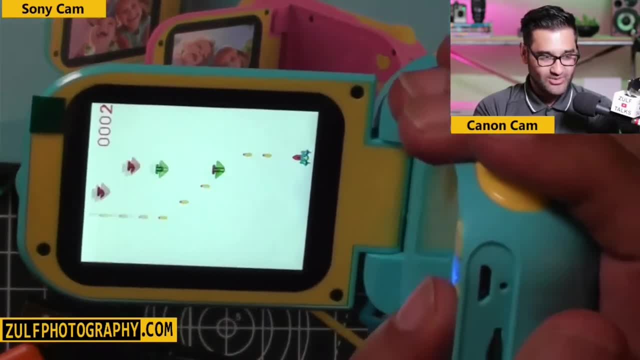 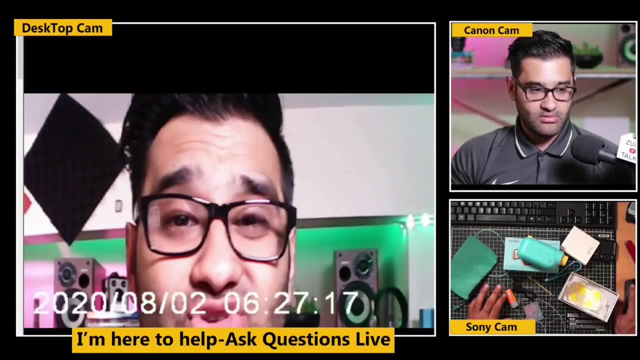 a little game on that. So look at that. It's a bit weird where the controls are because they're here, But Oh, I lost. But yeah, it's like a space raider, Space invaders kind of. Oh, The land yard took me ages to put in, But it's that camera. I haven't put the stickers on it yet. 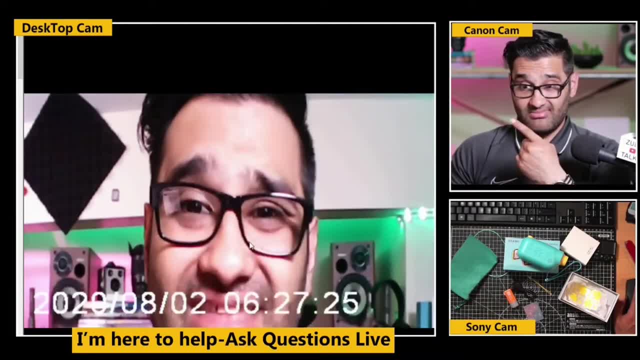 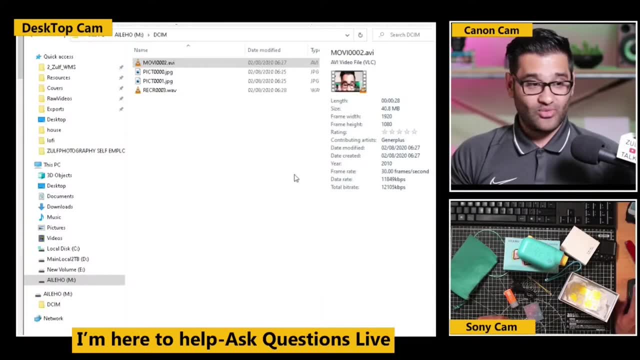 I'm at 1080p video quality. What does the mic sound like? That's the main thing I'm interested in. So, yes, Test video done. Okay, That is Check him out. So basically, I recorded that on this camera. 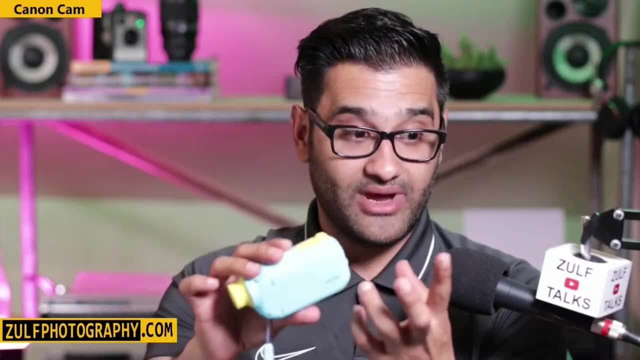 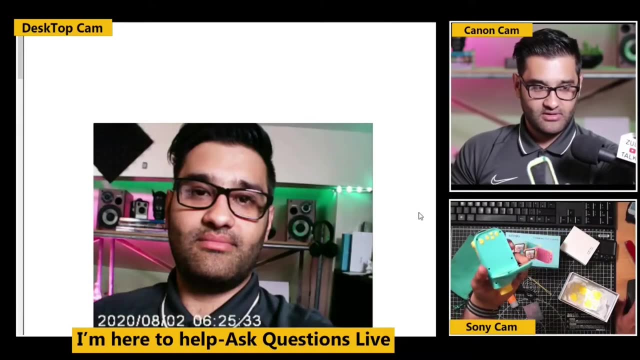 And I just played it back to you. It wouldn't play back on the device, which made me think it was bugging out, But it wasn't. Let's have a look at the pictures. actually. So that's the camera photo on this camera. So that shows you what it looks like And it's a VGA quality. I. 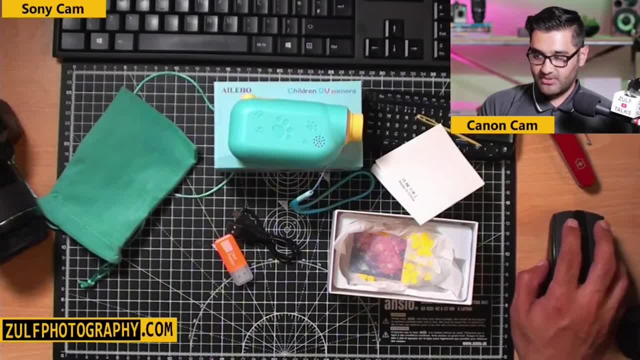 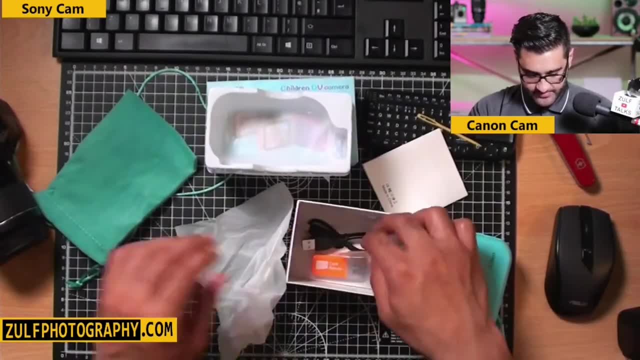 can't change that, So let's eject it from the computer. Always eject your cards correctly, because otherwise they corrupt, Because I can test that footage afterwards. Too shabby So far. What is my favourite? There's too many. There's too many here. 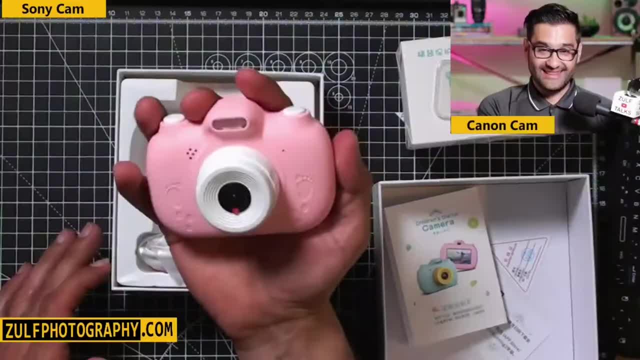 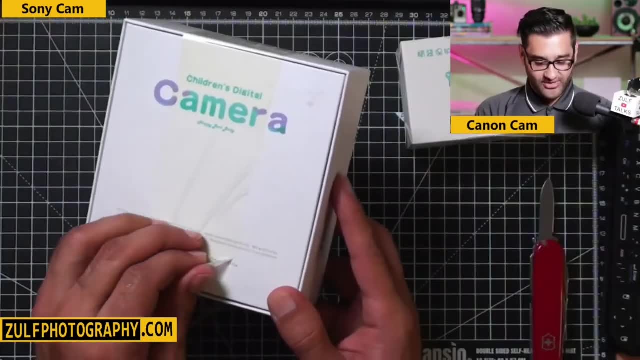 Okay, Let me put that back in. It's not that And it's not that. That's the size I was hoping for Touch screen. Look at this and see what it's. Give him a pink camera and he goes into school with. 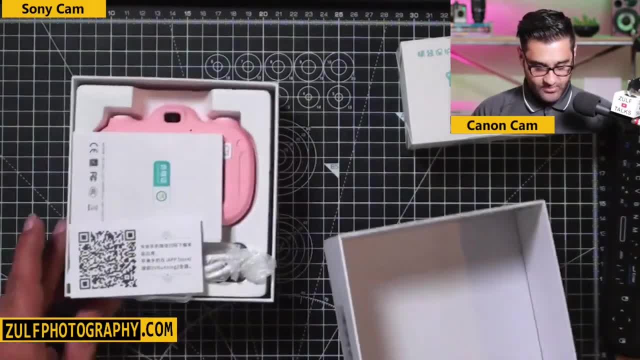 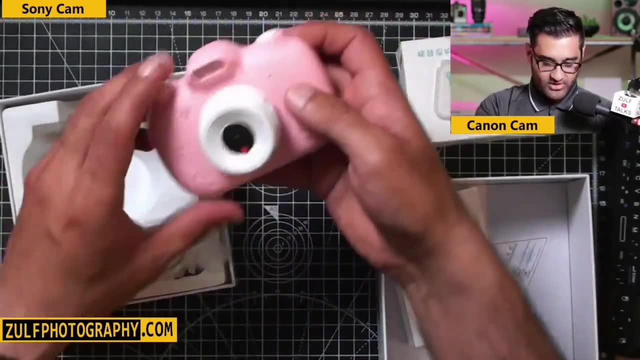 this. I'm trying to take the tape off without ruining the box. That is better. Oh, That's the size I was hoping for. If you remember the other one I looked at, it was smaller than this. So what does this come with? It comes with the camera. 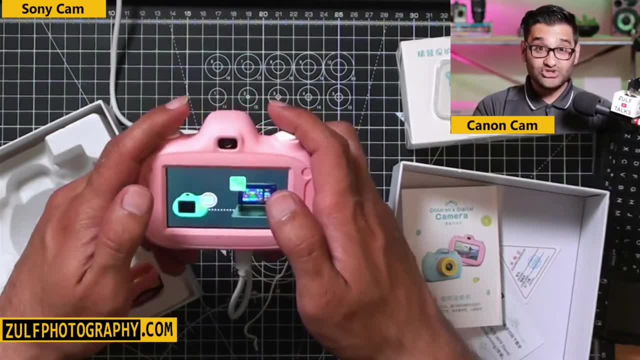 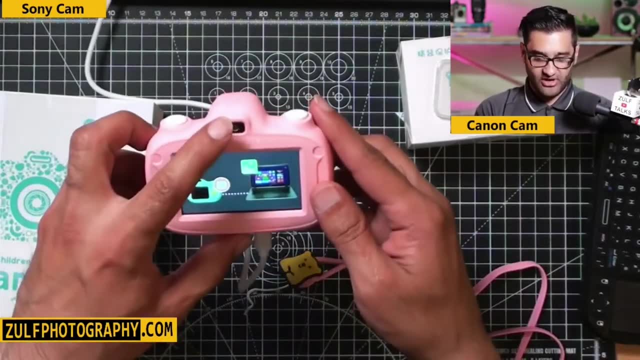 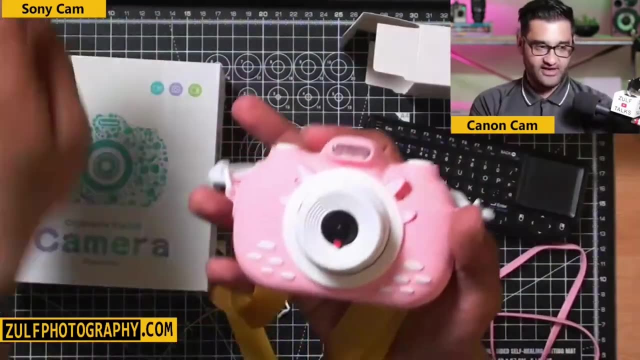 This is more serious: Touch screen. The lanyard quality has improved here. Okay, That has an eyepiece there, But actually that eyepiece does not work. So it's not You have to. I always keep one long nail just for that purple. You didn't just? Oh, no, man, Piece of kit. So now let's actually look at the menu. 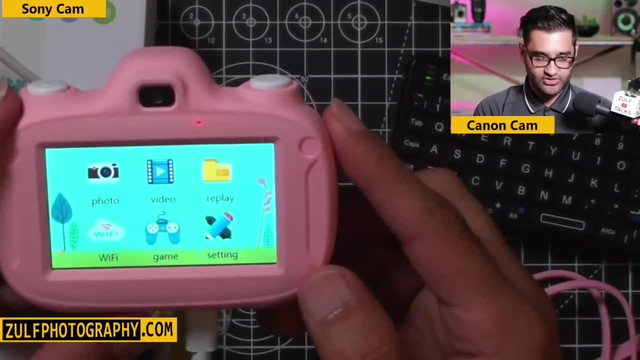 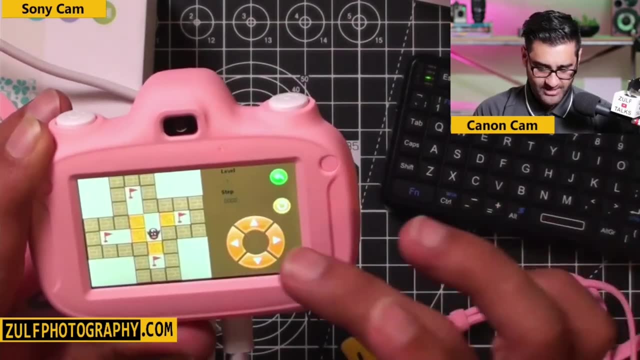 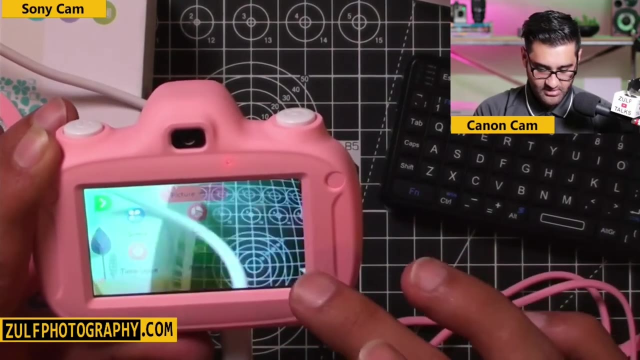 So we got photo. We got on switch, So I have plugged this into the charger right now. Okay, I Go to video. There's only one game: Scene colour, sequence, time lapse: Wait a second. Regular doubts. 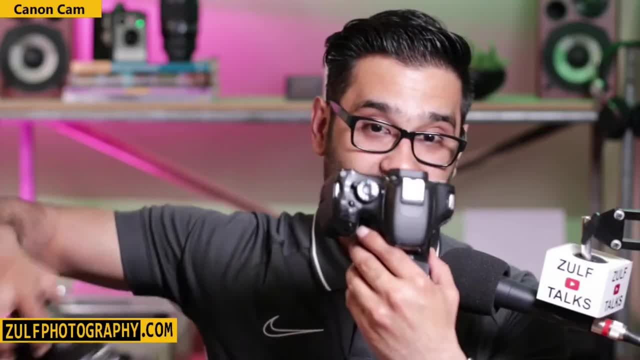 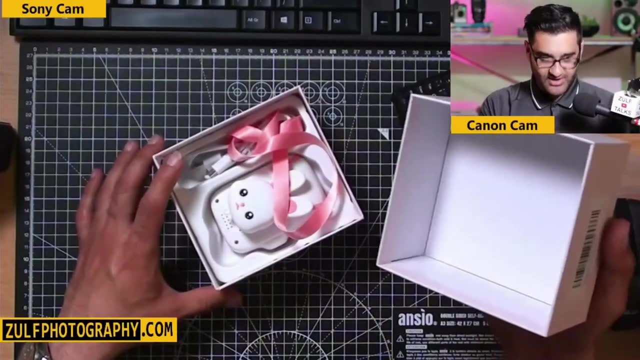 There's a lot more on there I can show you, But it's not that And it's not that. Oh, That's the size I was hoping for The kids. There's one, There's one, There's one. whoa, whoa, whoa, whoa, whoa, whoa, people, people. this is what it's all about now. 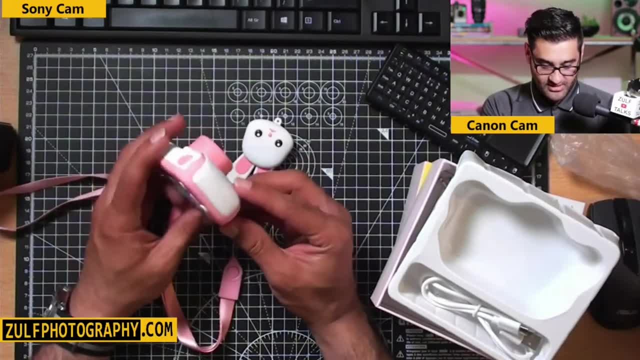 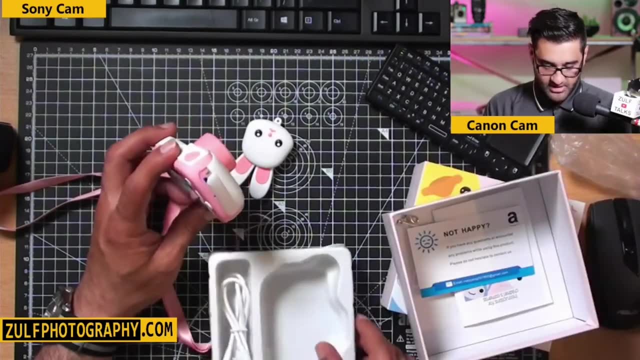 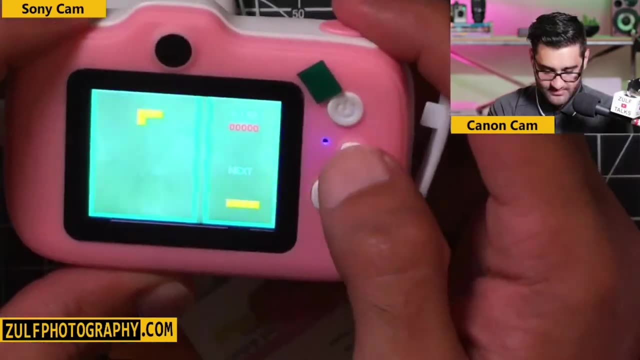 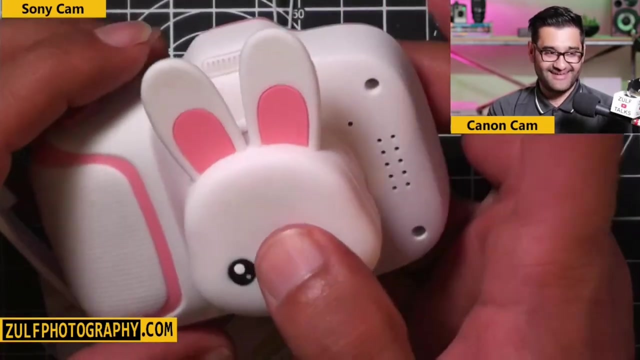 this one looks like. so it's got a little flap on the side. you'll charge it and you've got a memory card, which i don't think comes supplied. snake, pushbox, tetris, hey, hey, photo, there's no memory card. oh okay, internal memory. yes, whack it, mate. 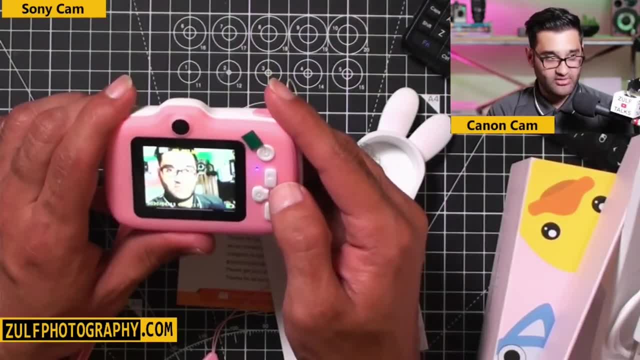 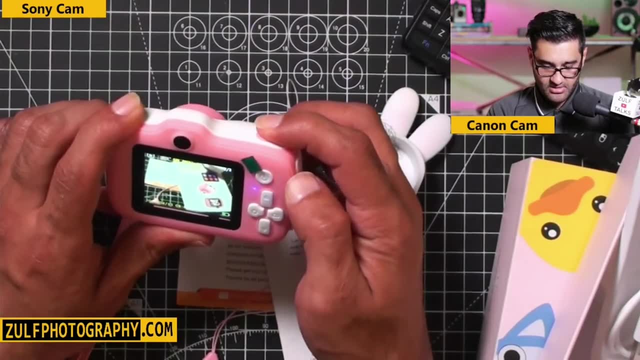 there's one. there's two camera's. not too good on it, but the game was better on this one. we can do some proper shooting with this. i'm gonna do that. okay, let's get rid of that. goodbye, bye, bye. do you have a little present for your kids? 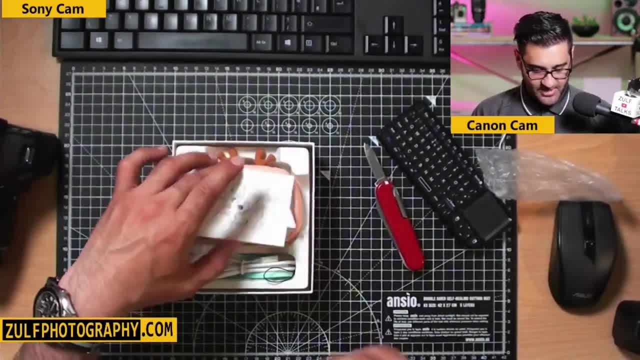 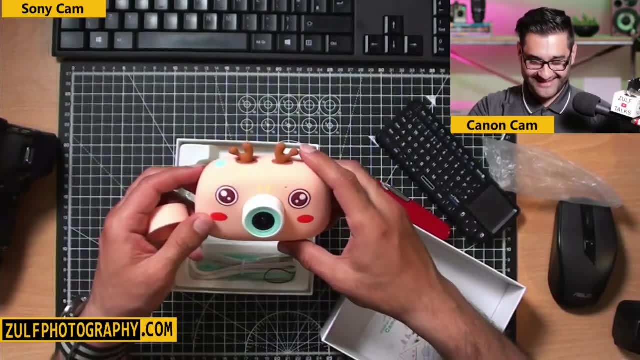 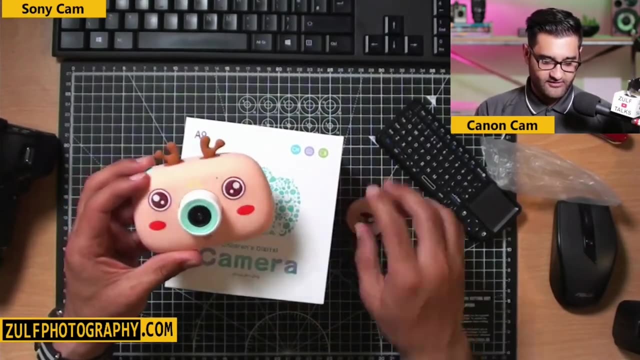 you. let's have a look at this one and see what it's all about. wait a minute, people. whoa, whoa, whoa, hey, hey, that's what i wanted. okay, you know what this case up there you can see it's got its silicon bit there. i'm gonna take that off. i. 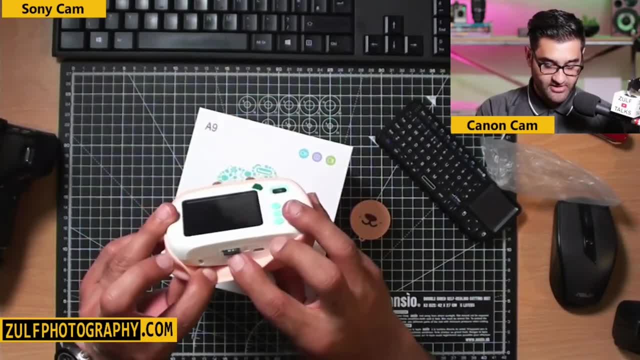 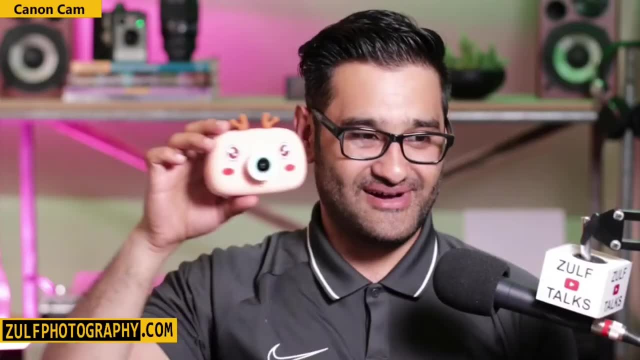 can see a little mic there, maybe a speaker, which is actually got a memory. it's got a memory card already in there. 18 megapixel camera. let's go to settings. there's a picture. what do you think of that? there's a smile to your face. look at that camera. 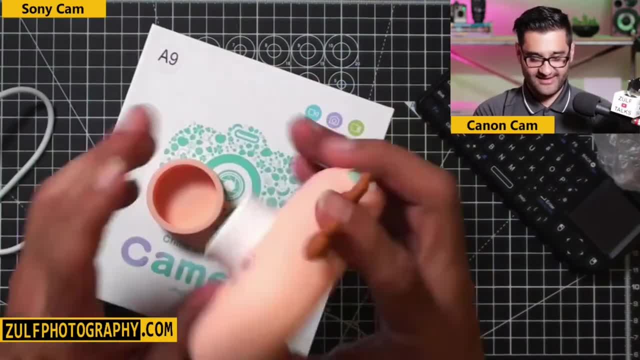 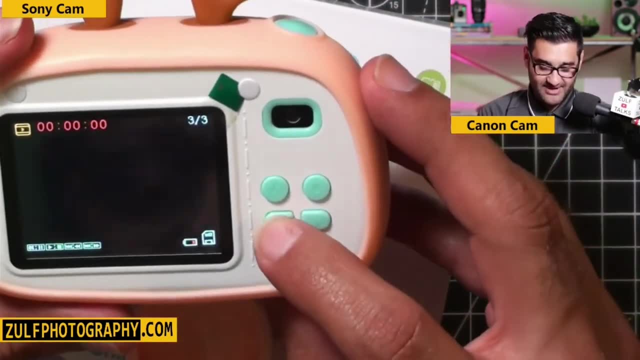 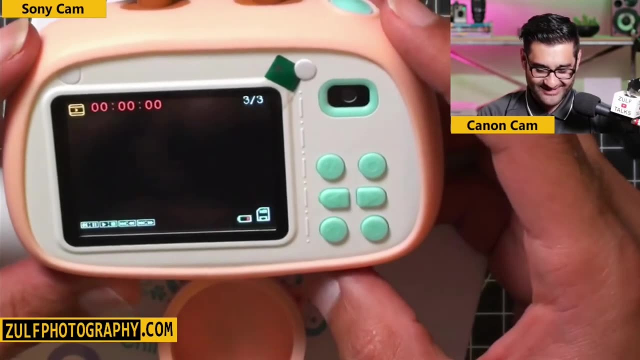 basically take that off. you've got your little lensy. see, this is. this is when you buy a camera- new- and each camera has its own menu. a bit frustrating, but you're seeing it. you're seeing it exactly so that one is not as robust as the other ones. what do i do now? how do i reset it? 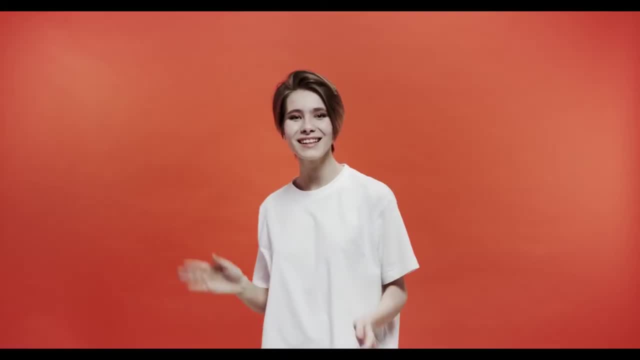 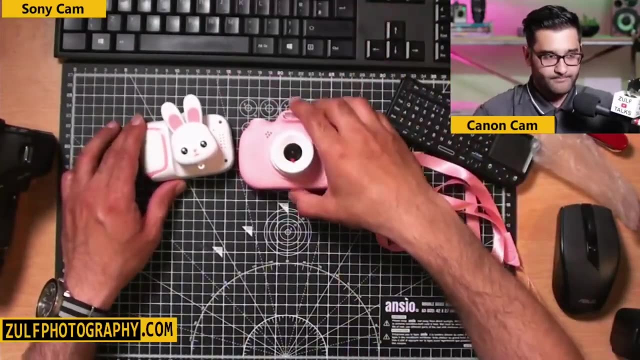 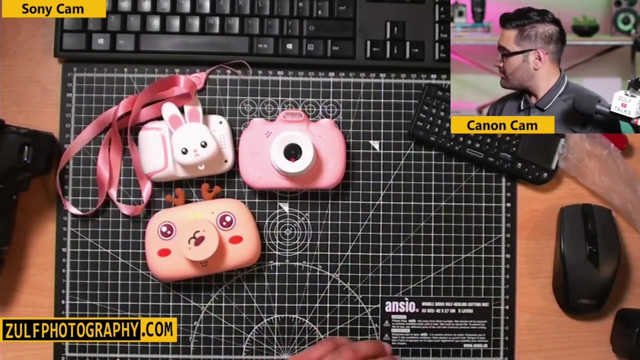 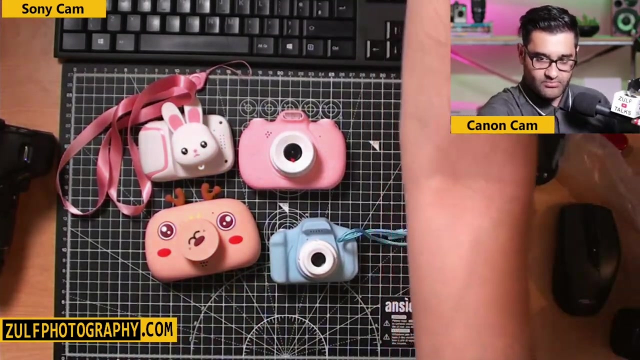 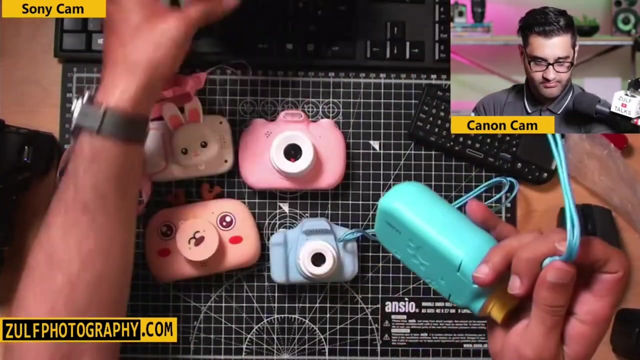 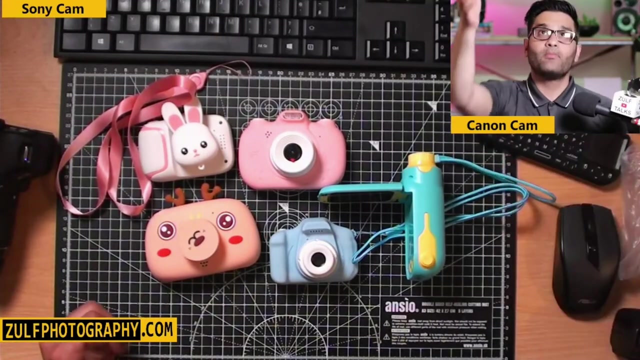 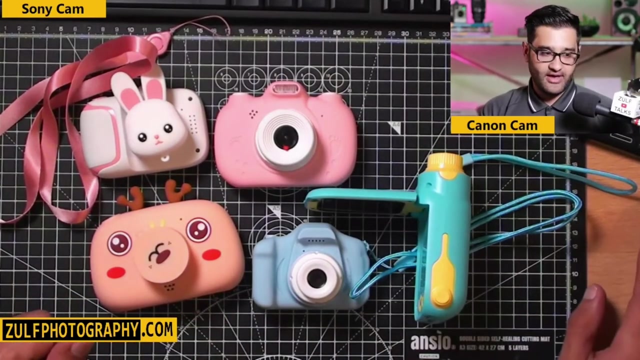 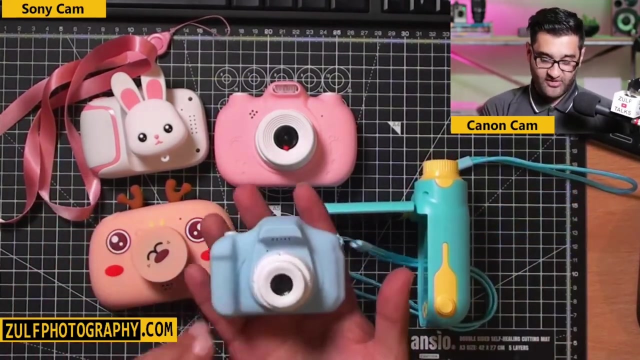 we'll have to read the guide. so so, so, so, so, so so there's one, there's another one here, so so okay. so if your series about photography and you want your kids to get a little gift idea, there's a number of cameras here. you can see from the small and cute. 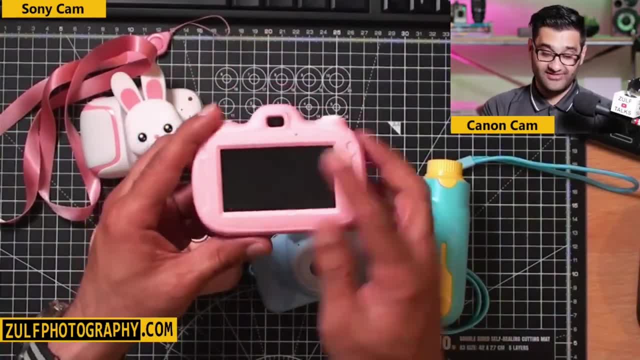 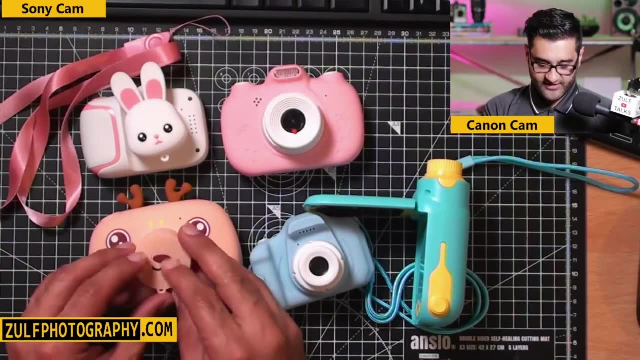 to the small and actually quite decent that has a touch screen on it and it's actually got games in there as well. so there's a few options here. you can see they have little cute lens caps, like that reindeer face is one and obviously we've got a rabbit one there. 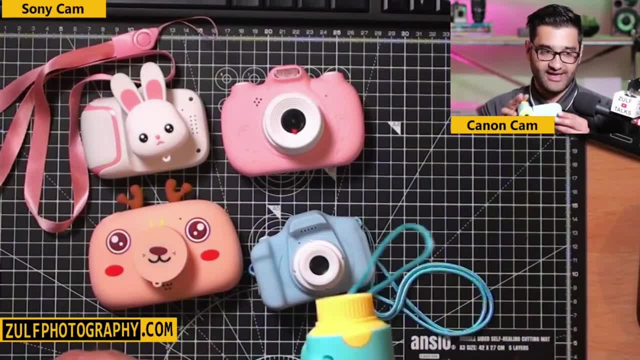 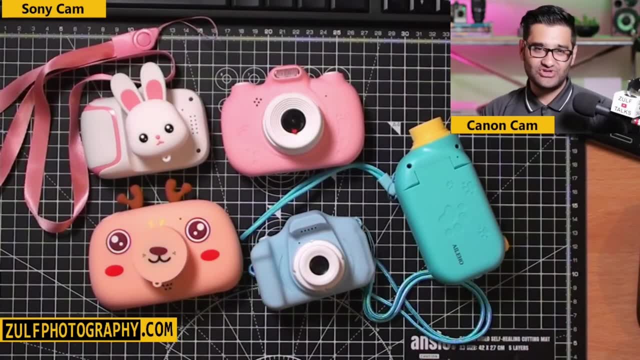 so we've done a couple of testing on this- more of a camcorder style one here- and you can see these are all little options for you to get shooting, basically photos, even video and games as well. so hopefully you found that interesting. i did a full unboxing. 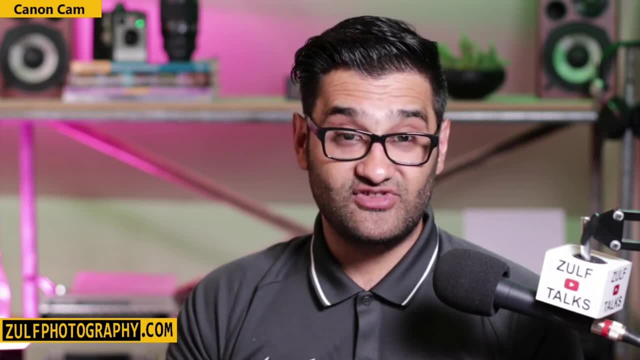 you can watch the full replay of this. chapters will have the breakdown and you can see if these are worth buying. take care and i'll see you in the next live.